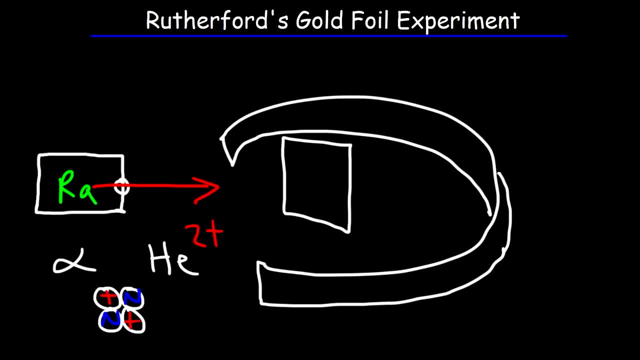 detector was coated with a fluorescent substance, so when the alpha particles were to hit it, it would flash. Now what he realized is that many of the alpha particles went straight through the gold foil. However, some of them bounce back, while others were deflected at large angles. 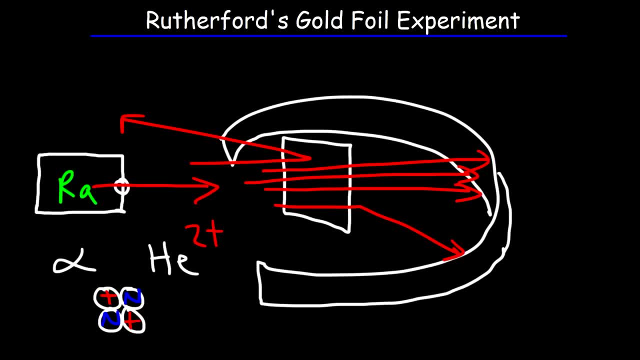 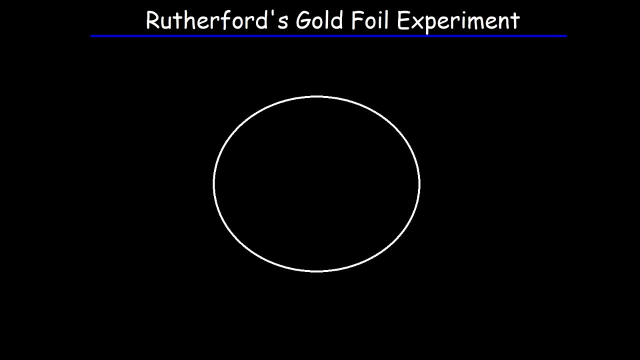 And so he came up with some very important conclusions based on what he saw, and he realized that the Plum Pudding model couldn't be correct. Now let's talk about some of those conclusions. Imagine if this circle represents an individual atom. The fact that most of 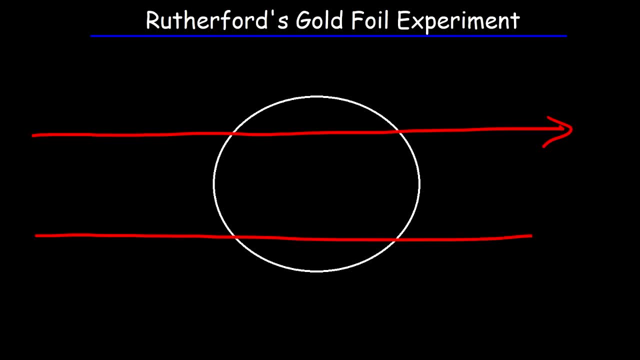 the alpha particles went straight through the gold foil. What conclusion do you think Ernest Rutherford came up with? Since most particles went through the atom or the atoms of the gold foil, he concluded that the atom must be mostly empty space. Now there was something else that he came up with: The 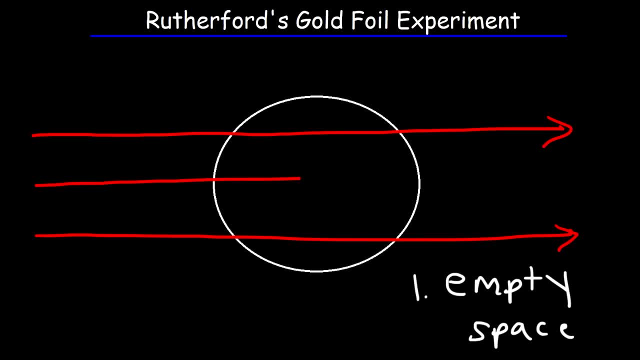 fact that some of the alpha particles bounce back, he realized that there must be a very dense center, which we know to be the nucleus. The second thing that he realized is that some of the alpha particles, they were deflected at large angles. 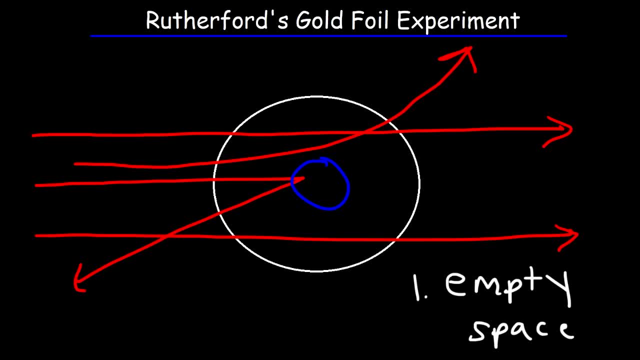 Now remember, the alpha particle consists of two protons, two neutrons. So the alpha particle has a plus two charge. Now we know that opposite charges attract. If you have a proton next to, let's say, an electron, these two, they're going to feel a force of attraction. But like 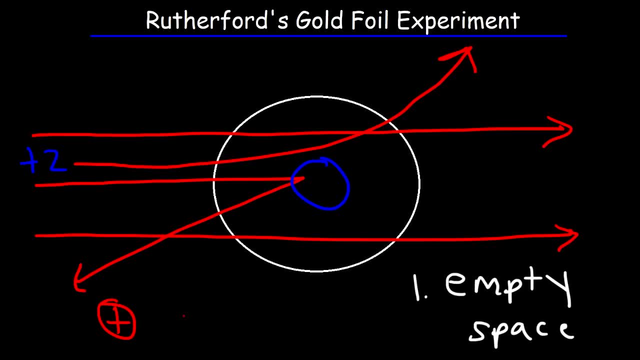 charges. they repel each other. So if you have, let's say, two protons next to each other, they will feel a force of repulsion, And so they're going to move apart. Now the fact that some of these alpha particles were deflected away from